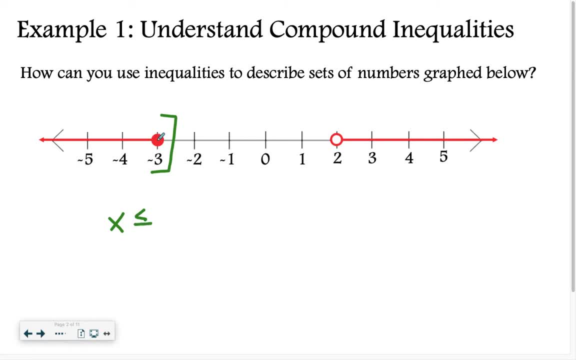 variable is less than or equal to, because that circle's filled in, negative three. And if I look over here, I have x is greater than not or equal to, because it's not filled in, and the number's two. So my question to you is: can a number be less than negative? 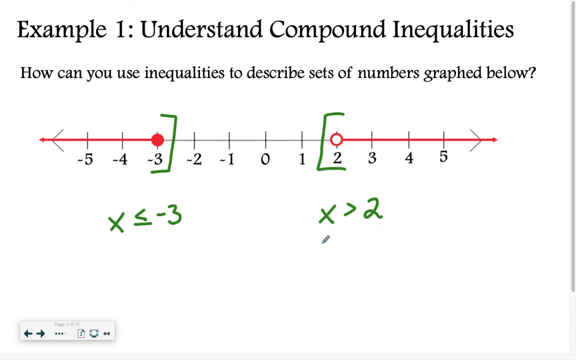 Three and greater than two at the same time. No, So what you're going to use is the word or. Whenever you have two graphs kind of happening at once and they can't happen like together at the same time. that's an or- okay. 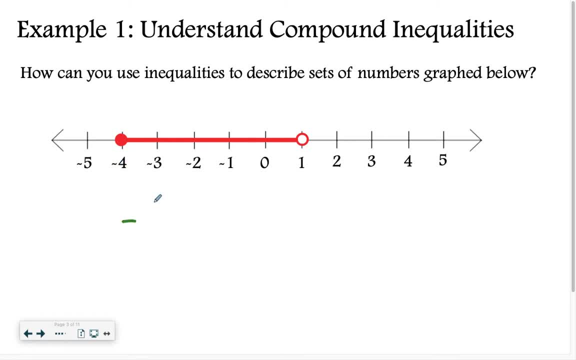 This, however, is a little different. So you can see, I have something at negative four, I have something at one. So if I were to ask you to describe this, you would maybe say, hmm, it's greater than or equal to negative four. 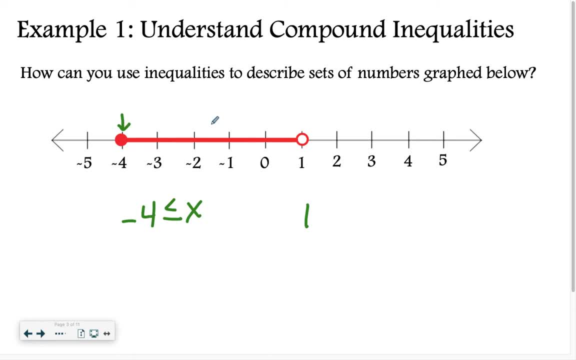 So I'm going to use a variable. But if I follow that shaded line, it's also. it stops at one. So it is also less than one. So the way you can write that is negative four x- sorry, I keep saying so, my apologies. You can write that saying negative four x is less than or equal to x. 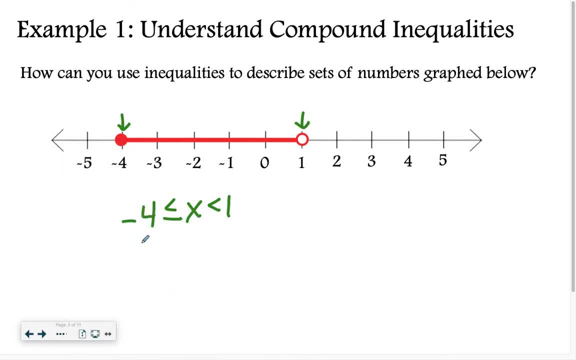 less than one. This is one possible answer that you can use to write that compound inequality. Or some people feel more comfortable saying it is negative four is less than x, And we have x is less than one. That's another appropriate answer. Some people- oops, that was a terrible box. Some people prefer to say x is greater than negative four. 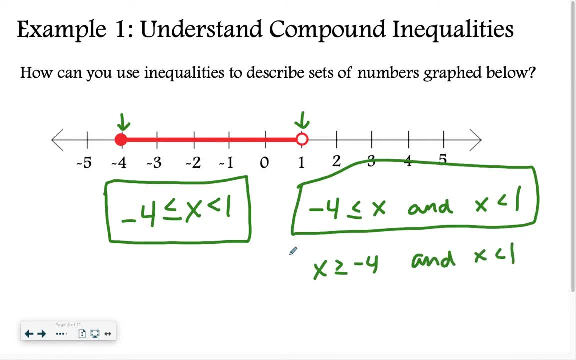 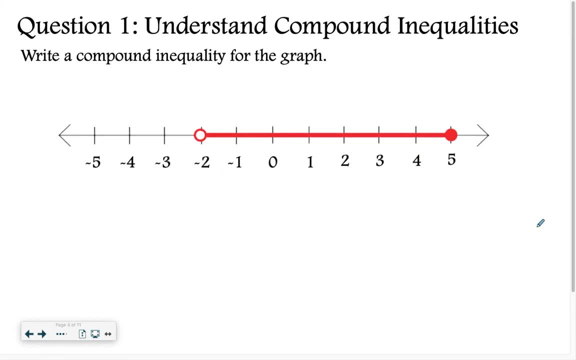 And x is less than one. Those are all correct answers. Everything that's boxed is an answer I would accept. okay, Now I want you to go ahead and try to write the compound inequality for this graph. Good luck, Hopefully. you said on the left side it is a negative two. 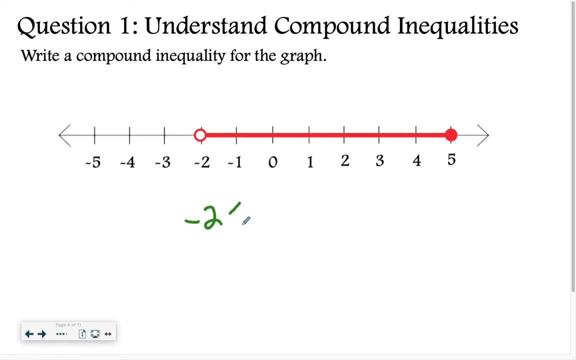 And I'm going to say that x is greater than Negative two, but x is also less than or equal to five. So this is one possible answer And I think I forgot to kind of mention on the last slide. whenever you have like something that has an end point on each side. 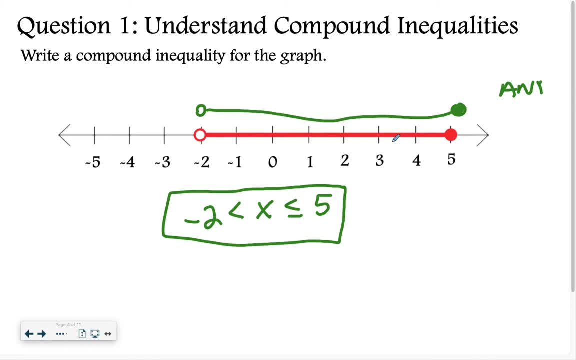 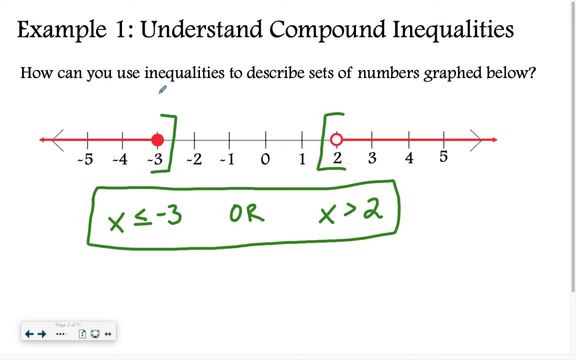 that is called an AND compound inequality. If I go back, you see how in this example the numbers kind of point out: Whenever you have that you're going to have a compound inequality. If you have that situation, that's called an OR. 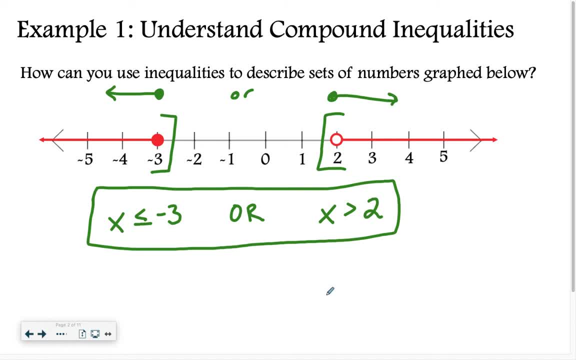 And one way I remember that is if you were trying to row a boat. okay, So imagine a rowboat. You have an OR on each side. The ORs have to stick out of the rowboat in order for the boat to move. 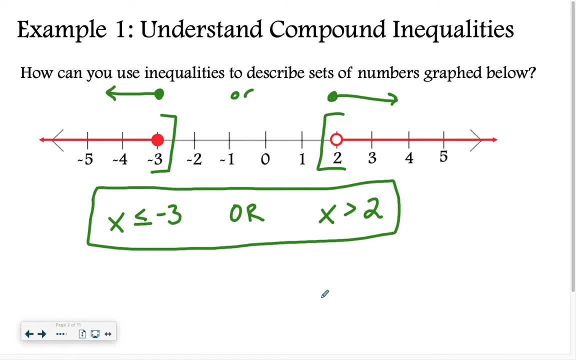 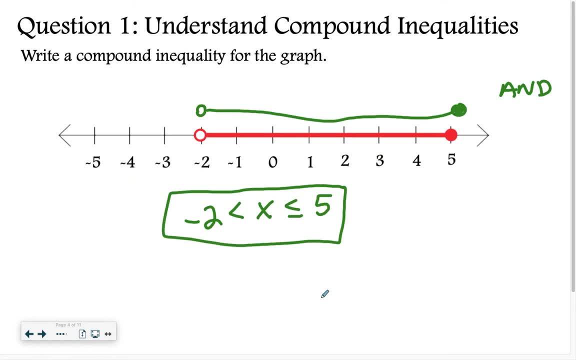 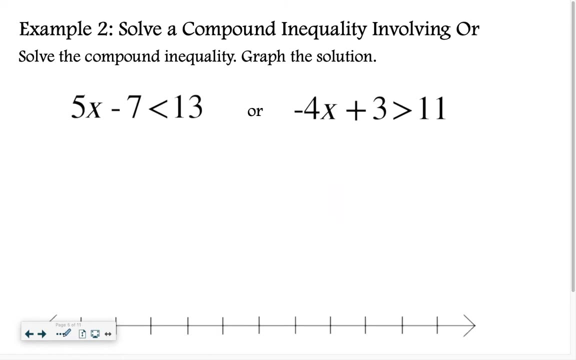 So that's one way I help myself remember that OR points out AND is when you have two end points and it's filled in between, Okay. So hopefully those couple of things will help you Keep track of AND versus OR. Now let's talk about just solving. 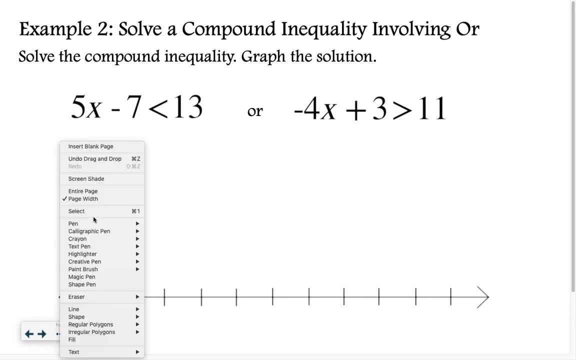 So we have an OR inequality here. We have: 5x minus 7 is less than 13, or negative: 4x plus 3 is greater than 11.. You might look at this and say I don't know how to start. 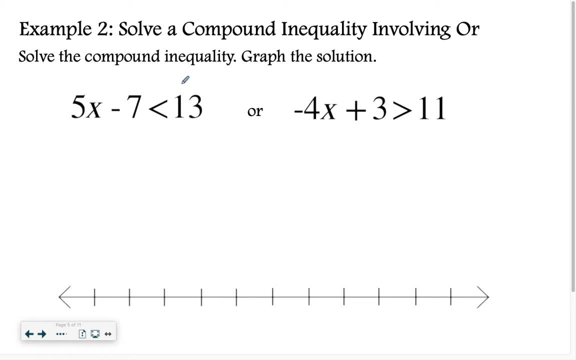 There's two inequalities. Well, it's pretty cool Because you solve them Just the same way. It's like you're going to solve two different inequalities. So I'm going to start by adding 7 to both sides, So I have: 5x is less than 20.. 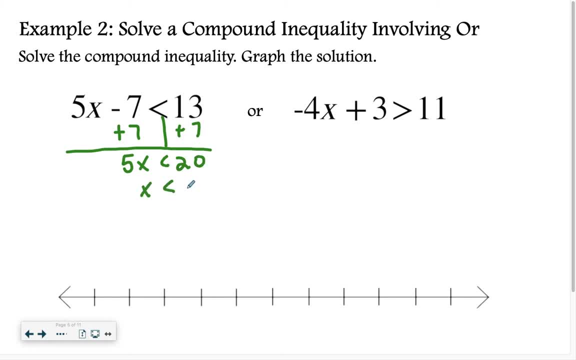 Then I'm going to divide both sides by 5.. So I'm left with x is less than 4 as one answer, And then I need to remember to write the word OR. Okay, so I start by subtracting 3 from both sides. 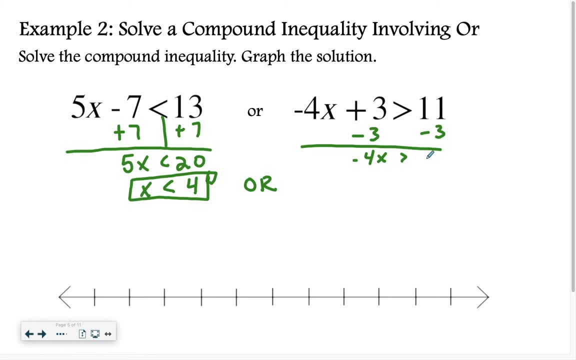 I'm left with negative: 4x is greater than 11.. I'm left with negative: 4x is less than 8. Then I divide both sides by that negative 4.. I'm left with x is less than, because I divided both sides by a negative. 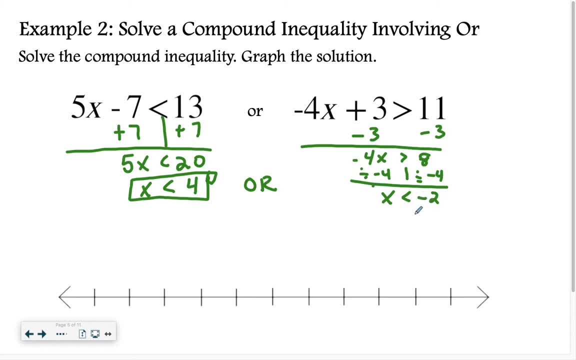 So I flip my sign And 8 divided by negative 4 is negative 2.. My two answers are: x is less than 4.. Or x is less than negative 2.. Okay, so now, if I look at this, I'm going to write: let's see, this can be negative 2.. 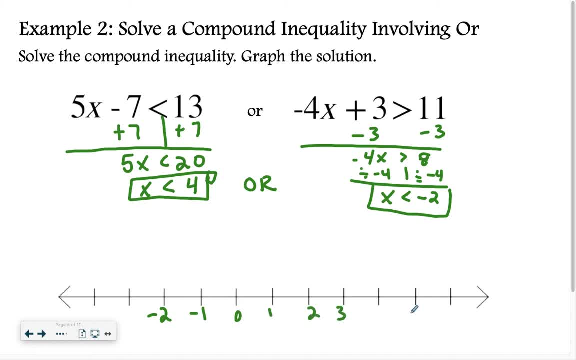 Negative: 1, 0, 1,, 2, 3, 4,, 5, 6.. Alright, so if I have x is less than 4, that's going to be an open circle at 4.. And that's going to go on and on this direction, right. 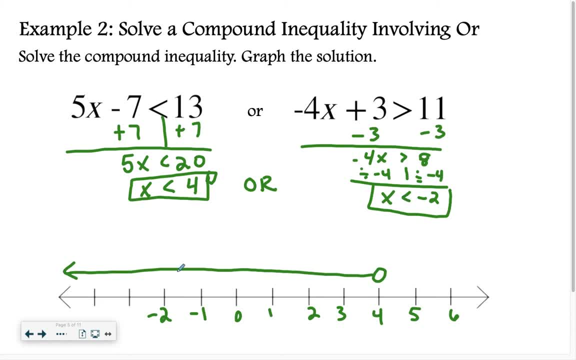 Then if I have x is less than negative 2, that would be an open circle Going like this. So you can see, sometimes people in rowboats get a little confused or they have to make a really sharp turn For whatever reason. pull the or in from one side and have both of them sticking out on. 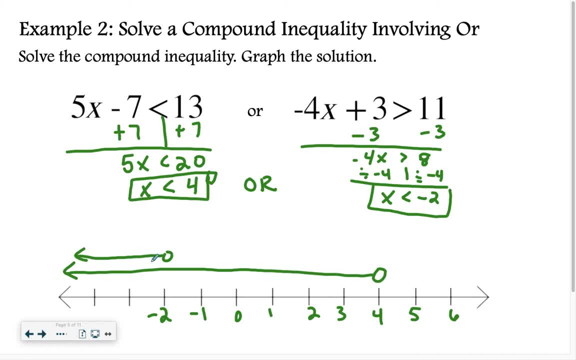 the other side. So or can also end up where you just have it pointing in one direction, Since the x is less than negative 2, do you see how this Overlaps? Whenever you have that overlap, you don't actually need to draw in that overlap. 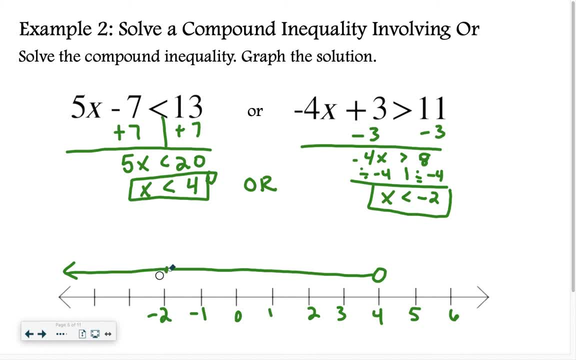 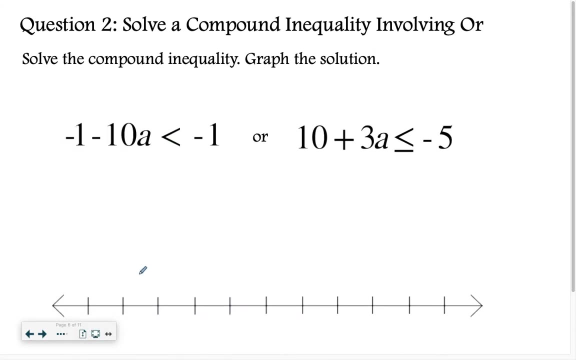 You can just leave it like this as a final answer. Okay, so that can be your final answer for that problem. I'm just going to switch back to pen. Alright, now I want you to try this problem on your own. Good luck. 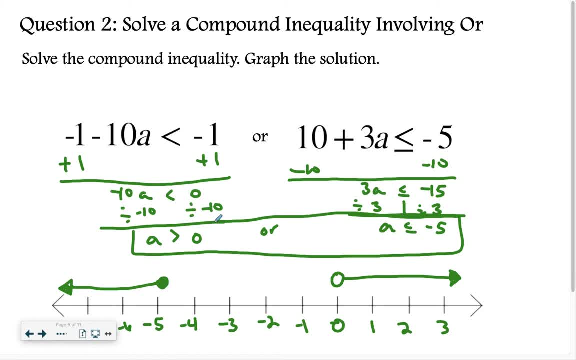 Okay, hopefully for this problem, you ended up with a is greater than 0, or a is less than or equal to negative 5, and then your graph looked something like what I have down on the bottom. If not, please don't hesitate to ask for some help. 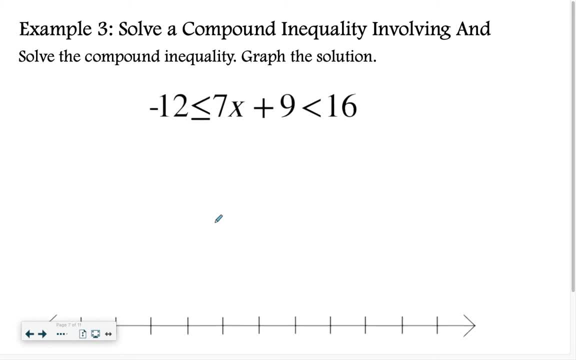 I'm more than happy to help you. Let's look at example 3.. So you can see that we have negative. 12 is less than, or equal to 7x plus 9 is less than 16.. You have a couple of options here. 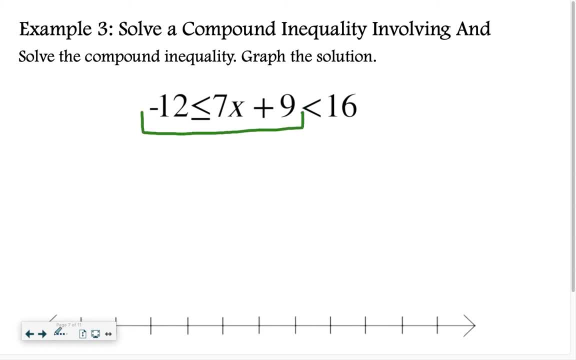 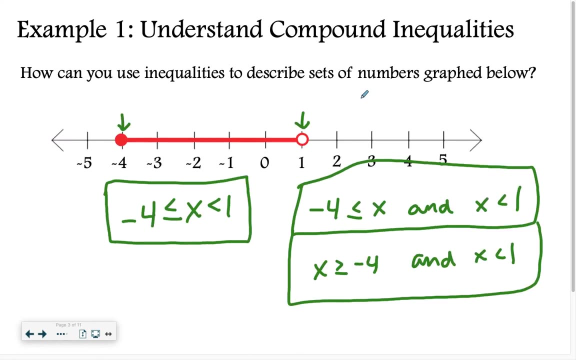 You can either split up this inequality into two parts. You can do the green part first and then you could do the purple part second. If you were to split that up, you would split it up and it would look something like nothing that I've done so far. 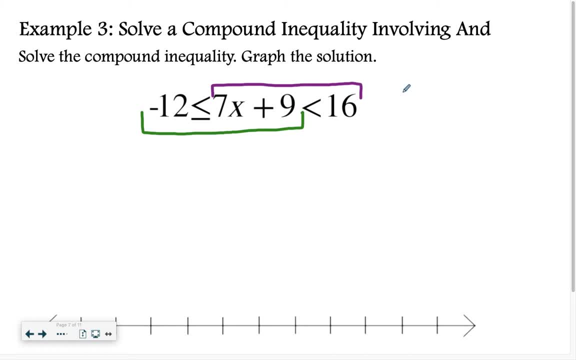 So let me show you what I mean. So I could split it up to be 7x plus 9.. 9 is less than 16.. And then I could split and just do the green separately. So I could say negative: 12 is less than or equal to 7x plus 9.. 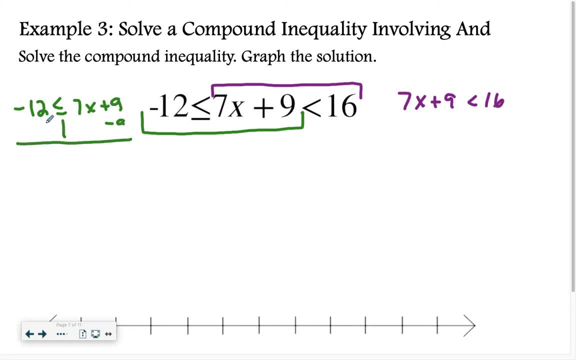 And then I can just solve from there. So what I can do is say minus 9. minus 9,, that's negative 21, is less than 7x. Divide both sides by 7.. Divide both sides by 7, that's a negative 3, is less than or equal to x. 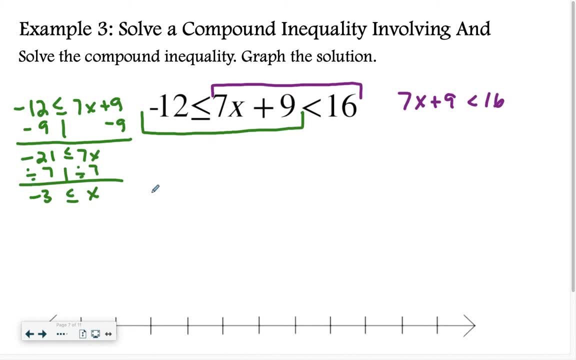 Since I divided by a positive 7x, I don't have to flip that sign. And then, if I move on to the one on the right-hand side, I would again subtract 9,, subtract 9.. So now I have: 7x is less than 7, or x is less than 1.. 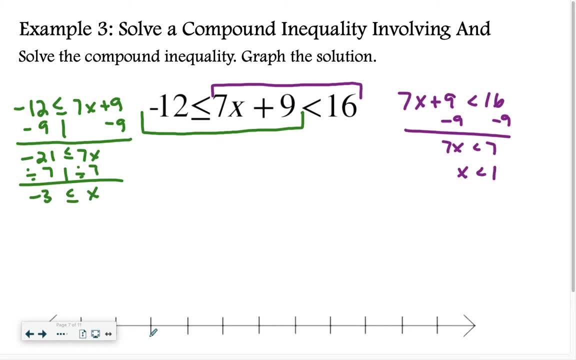 Okay, so a number is greater than negative 3.. That's what I get from the green, So I'm going to do a circle at negative 3.. Circle at negative 3, filled in because it's or equal to, And it is also less than 1.. 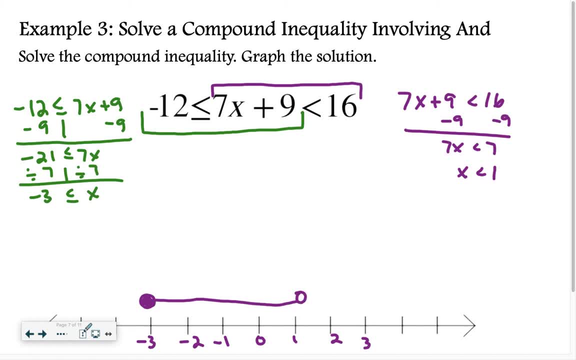 So I'm going to leave an open circle above that 1.. So that's one way that you can solve the problem. when it's written kind of all together like that, I know that can look a little intimidating. So if you want to split, by all means go ahead and split it up into two inequalities. 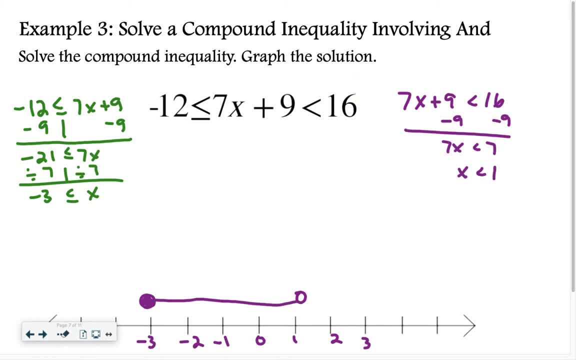 to solve. If you want a slightly faster way, here is one other way that you could do this. So if you want to split, by all means go ahead and split it up into two inequalities to solve. So if you want to split, by all means go ahead and split it up into two inequalities. 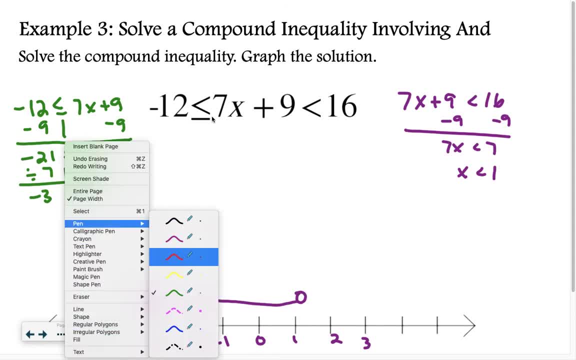 to solve. If you want to split, by all means go ahead and split it up into two inequalities to solve. So, if you want to split, by all means go ahead and split it up into two inequalities to solve. Here's one way that you could do this. 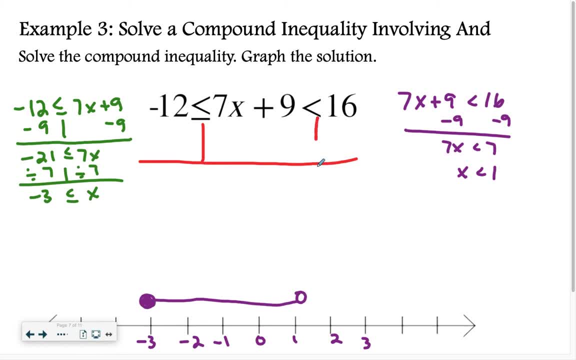 So I'm actually going to use a color I have not used yet. So what you're going to do is, instead of just moving it from one side to the other, what you're going to do is, if I subtract 9 from the middle, because I want 7x by itself, I 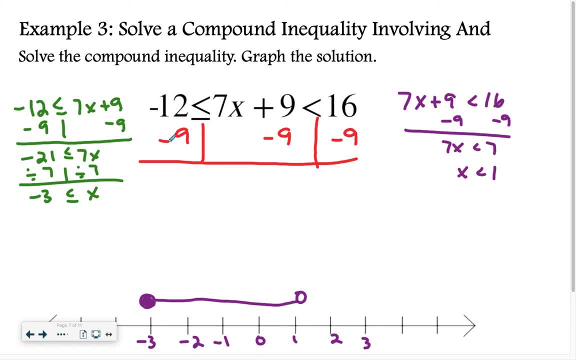 have to subtract 9 from every side of those inequalities, So negative 12 minus 9 would be negative 21.. We have is less than or equal to 7x is less than 1.. Okay, so now I have 7x. 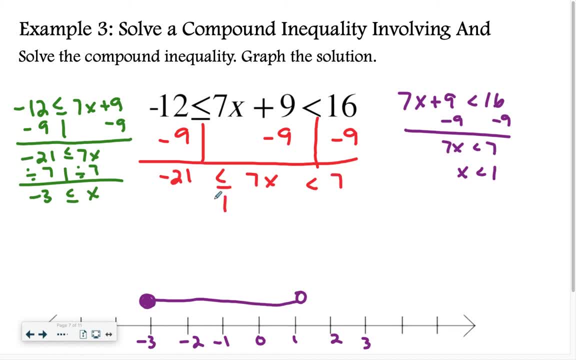 16 minus 9 is 7. so again, I draw the two lines from my inequalities. I say: okay, I have to divide by 7, divide by 7, divide by 7 in order to get X by itself, and I am left with negative. 21 minus 7 is or not minus divided by negative. divided by: 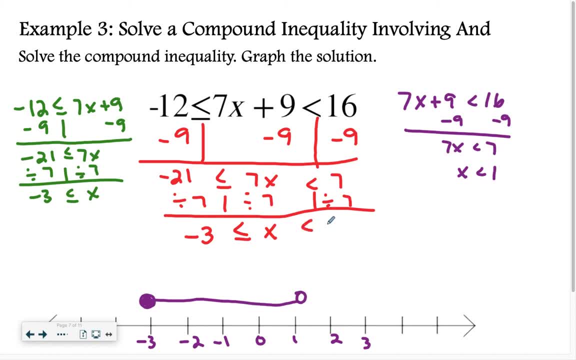 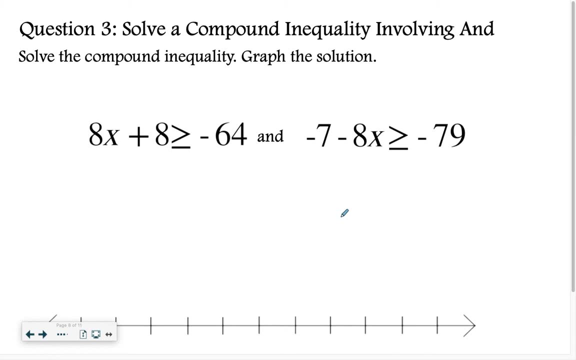 positive 7, my goodness is negative 3, and then 7 divided by 7 is 1 and that is how you can write your answer. all right, well, questions for you solved the compound inequality. then graph the solution. good luck, okay, hopefully for your answer you got. X is greater than or equal to negative 9. 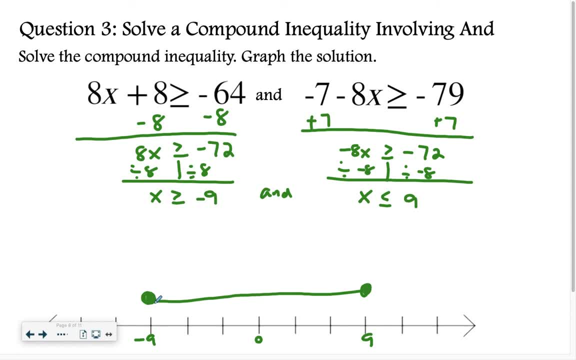 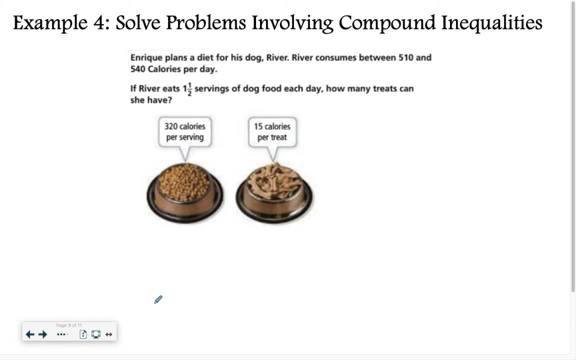 and X is less than or equal to positive 9, and then your graph looks something like what I have there. alright, let's look at our last problem, for our last example for today. a diet for his dog, River River, consumes between 510 and 540 calories each day, So we're going to 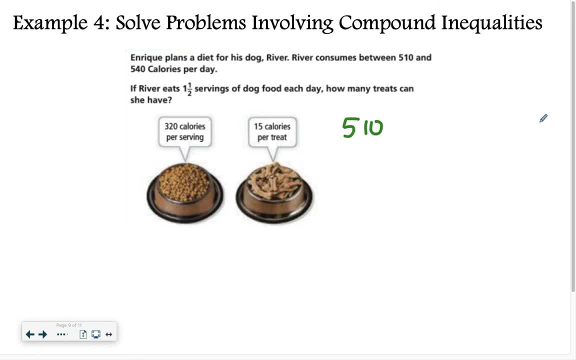 say 510 and then 540.. Okay, so we know that it's going to be either greater than or equal to that 510, or it's going to be less than that 540.. Now if River eats one and a half servings of dog food? 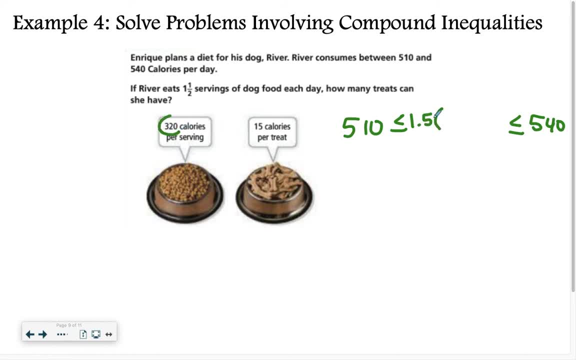 so 1.5 times 320 calories per serving plus. so that's how much his food is. We have treats and we know it's 15 times. I'm just going to do x to represent the treats. You can use a different.